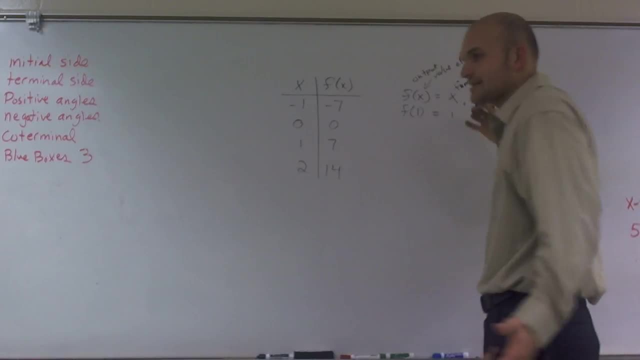 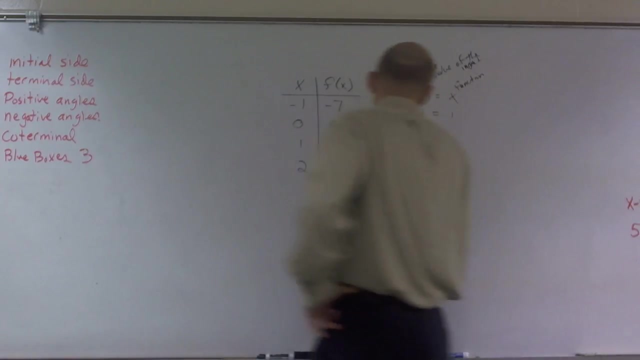 This is really what we call, just like the function, But it's also called like the input. But if I plug in 1, which is my input, I'm going to get out 1 for this function. But if I said like let's say, f of x equals x plus 2, and then I plug in a 1,. 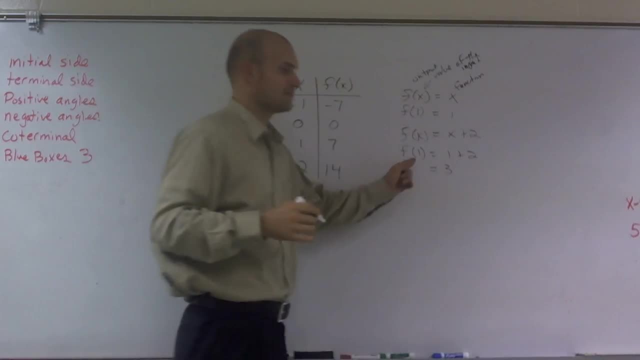 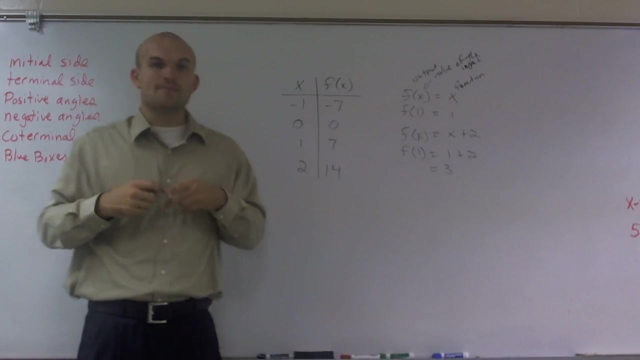 I would get 1 plus 2, which is equal to 3,. okay, So that's how you could get something different. If I had plugged in a 1, then I'd get out a 3.. So what we want to do is I always like to look at what am I adding and subtracting first? 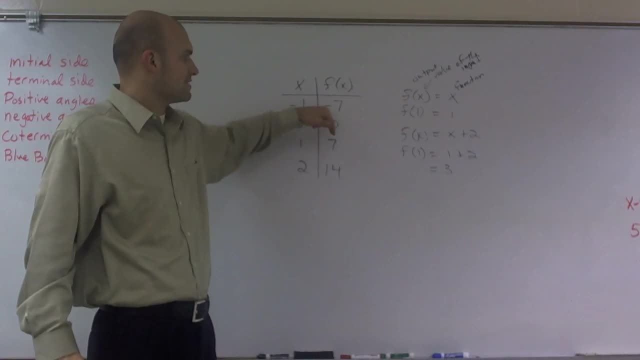 So I look at this to go from negative 7 to 10.. So negative 1 to negative 7, I would have to subtract 8.. And then what I want to see: is this true for the rest of them? Well, 0 minus 8 does not give me 0, and 1 minus 8 does not give me 7.. 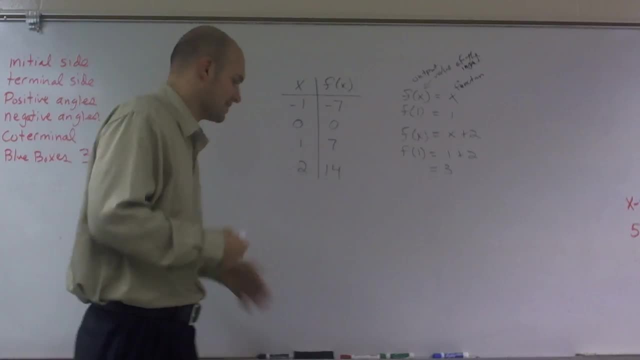 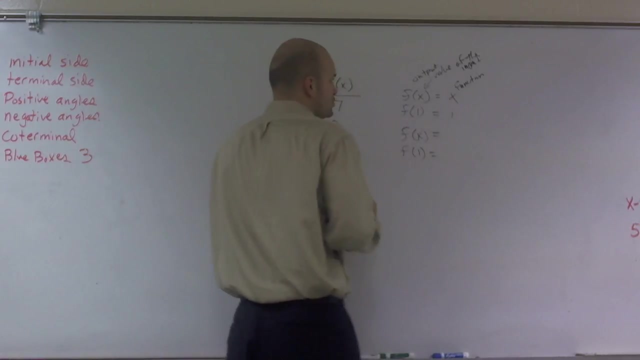 So therefore, subtracting or adding is not going to work. So the next thing I want to look at is what about multiplication? If I multiply a number, let's say, for instance, let's say my new function was 2x. 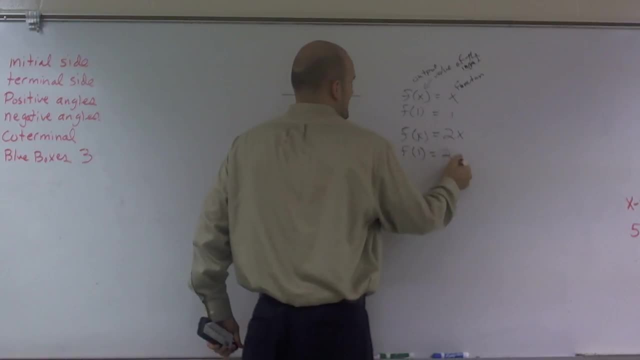 Well then, 2 times 1 would still actually give me 2 in this example, But if I did f times 3,, then I'd have 2 times 3,, which would leave me 6.. So I need to say: well, how could I? 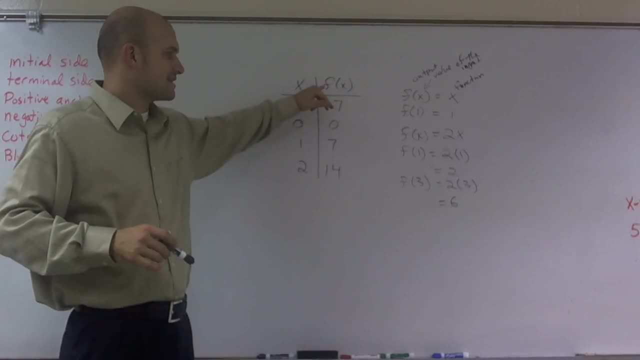 Can I multiply numbers to my x to get my f of x value of negative 7? Or to get my f of x value? So if I plug in a negative 1,, what do I have to do to get a negative 7?? 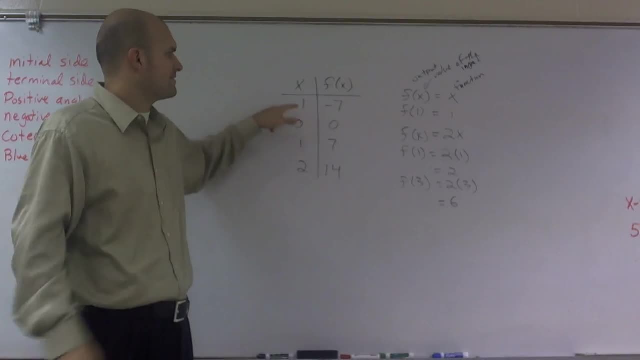 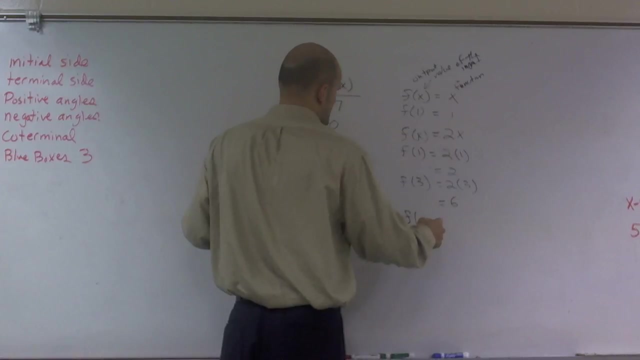 We already ruled out. you can't add and subtract, So what about multiplying? What do I have to multiply by negative 1 to get me negative 7?? You could say, well, you can multiply by 7, right. So we could say: f of x is equal to 7 times x. 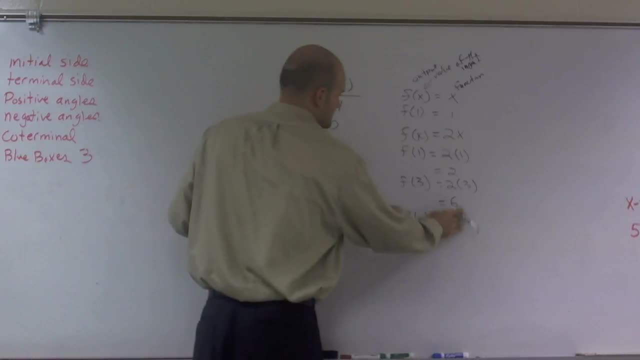 First we're going to do 7x, So we know that works for the first equation. Does that work for the next one? If I plug in a 0, f of 0 equals 7 times 0. Do I get 0 again? 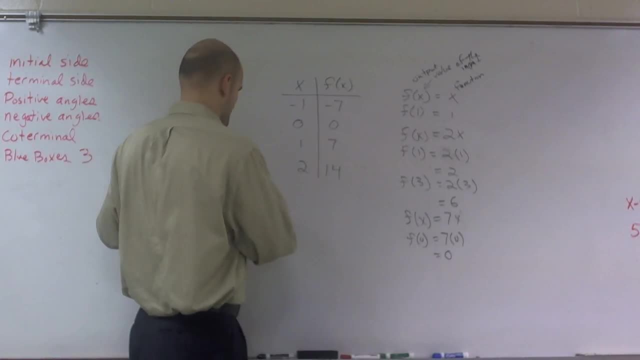 Well, 7 times 0 is obviously 0.. What about f of 1?? f of 1 is 7 times 0.. f of 1 is 7 times 0.. f of 1 is 7 times 0..